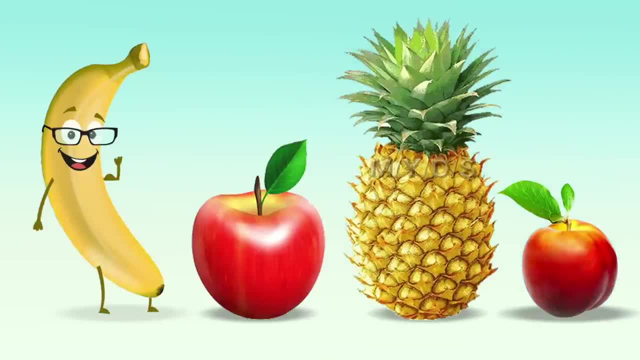 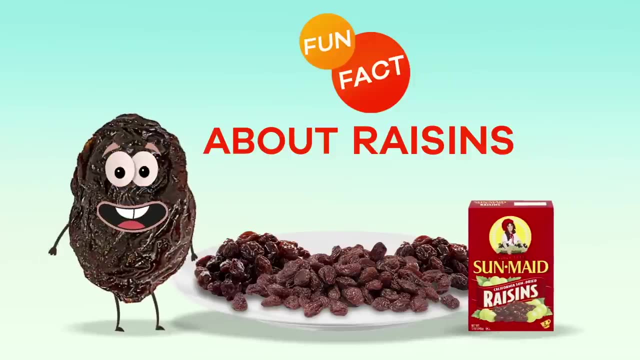 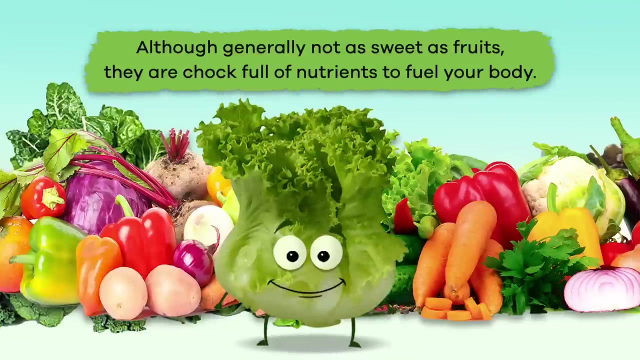 bananas to pineapples and nectarines. Fun fact: raisins are considered fruits because they are dried grapes. Cool huh Up next vegetables. Although generally not as sweet as fruits, they are chock-full of nutrients to fuel your diet. 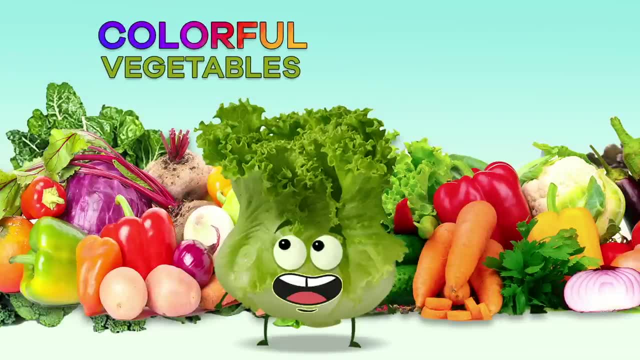 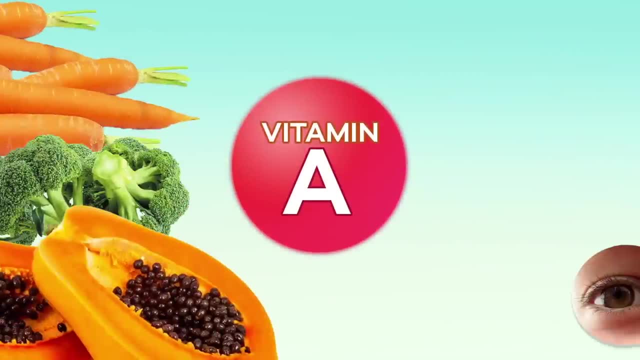 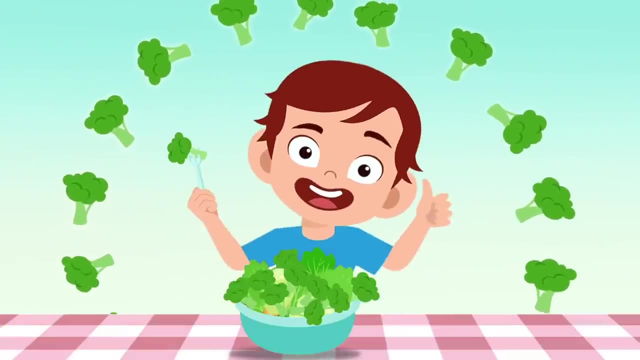 Here's a tip: The more colorful vegetables are, the more vitamins and minerals they have, Like vitamin A, which helps your eyes, white blood cells and skin. So the next time you wrinkle your nose at a piece of broccoli, remember that it is super good for your eyes, Fun fact. 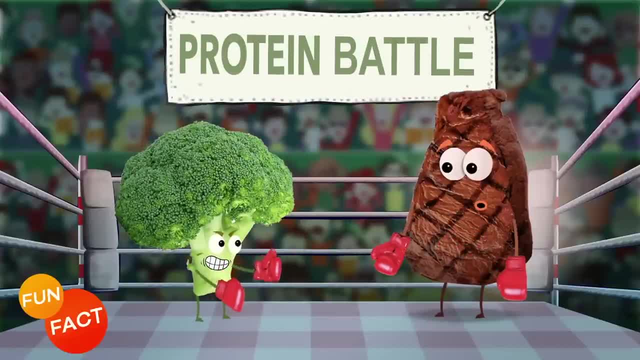 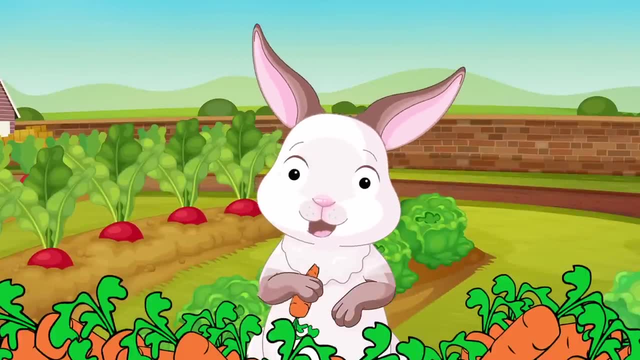 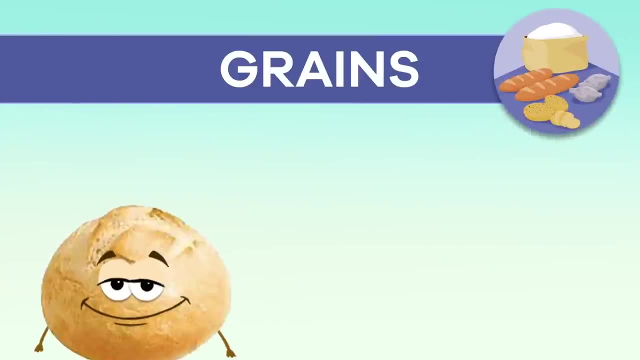 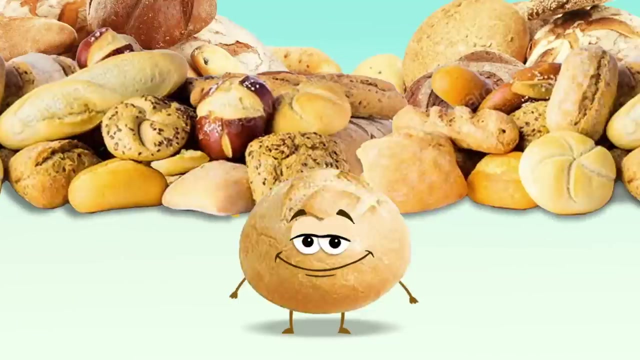 broccoli has more protein than steak Wild right. If broccoli is not your favorite, you can channel your inner bunny rabbit and feast on carrots, spinach and other leafy greens. Next, let's talk about grains. What food do you think of when you think of the grains group? Probably bread, right Bread is. 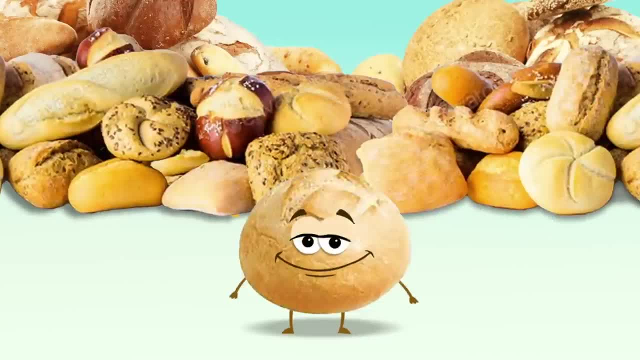 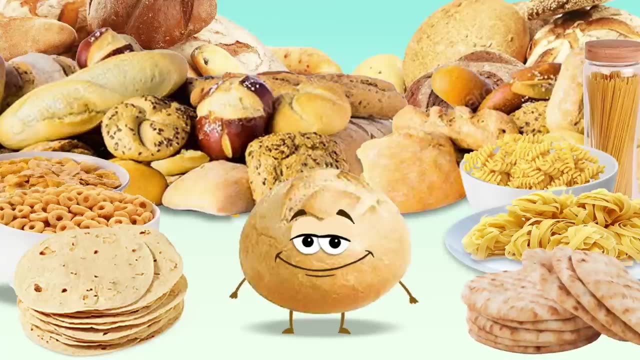 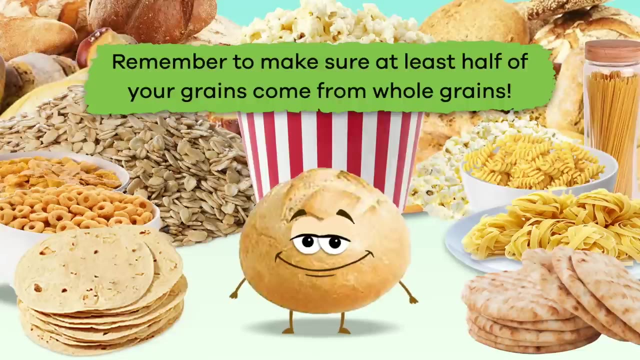 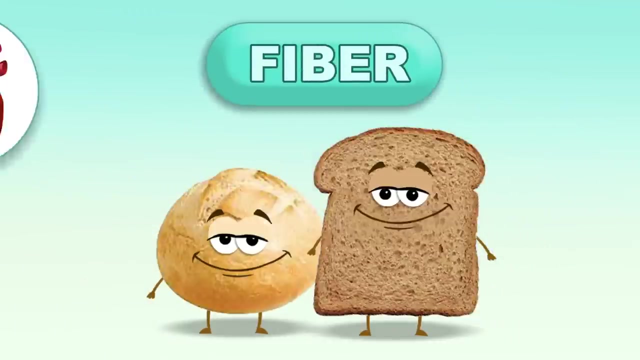 definitely part of the grains group. Other foods that are included in this group are cereals, pasta, tortillas, pizza, oatmeal, popcorn and many, many more. Remember to make sure at least half of your grains come from whole grains. Grains provide your body with fiber, which helps protect your heart. 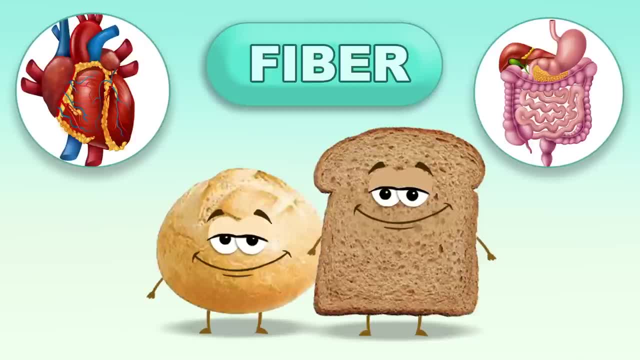 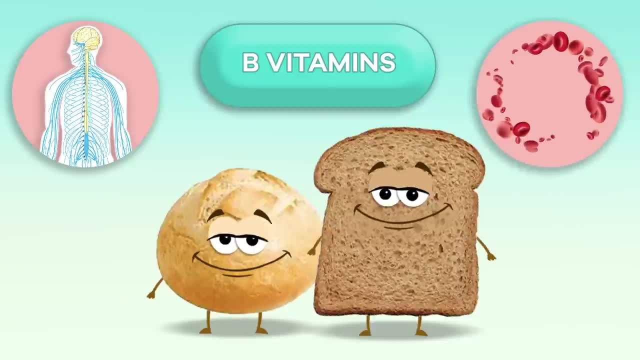 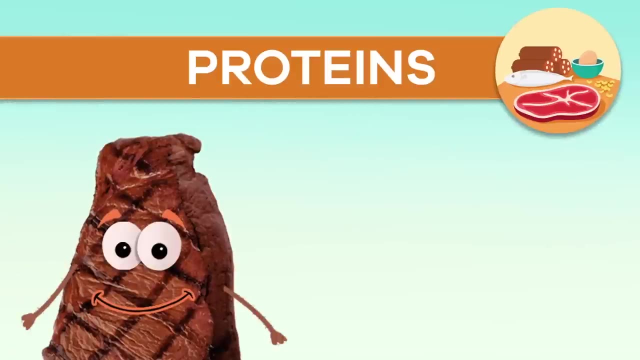 and helps your digestive system work properly. And the vitamin B in grains helps with your nervous system, the production of blood, and can help protect you from getting sick. Wow, Our next food group: proteins. Proteins might make you think of things like: 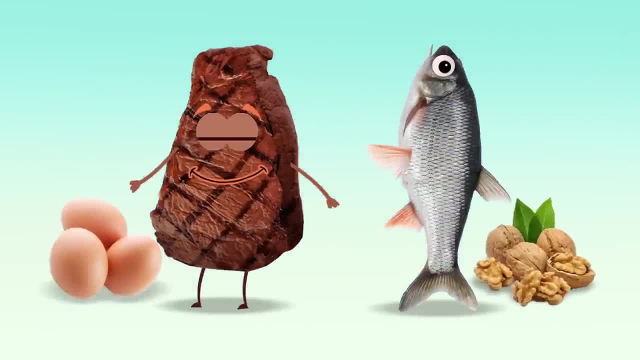 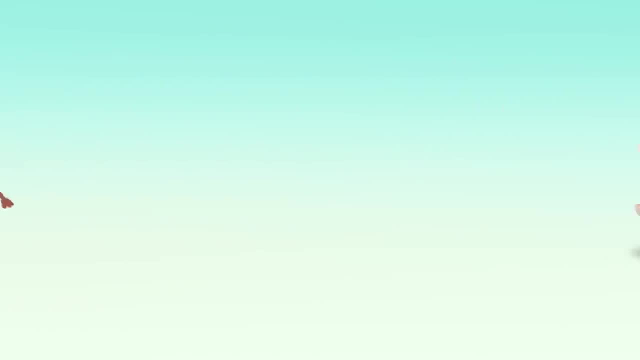 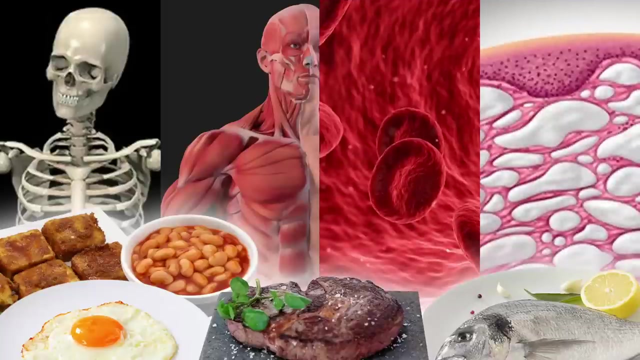 meat and fish, but eggs, nuts, tofu, lentils and beans are also part of this group. Protein helps with the formation of bones, muscles, blood and other tissues. Other nutrients found in this food group include vitamin E, vitamin B and vitamin C. Proteins are also part of this group Proteins. 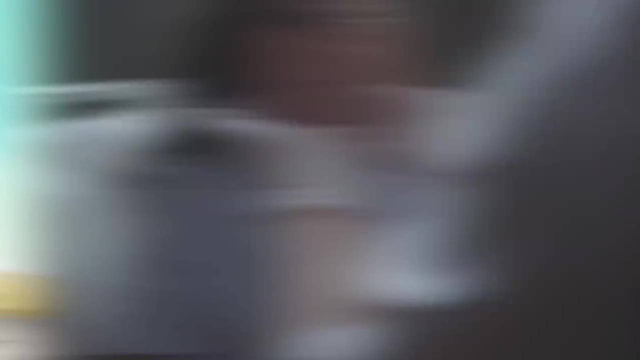 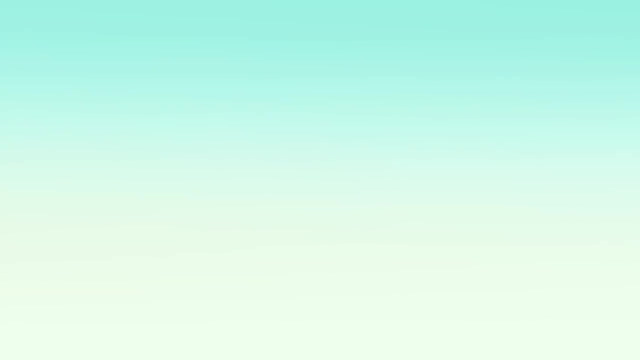 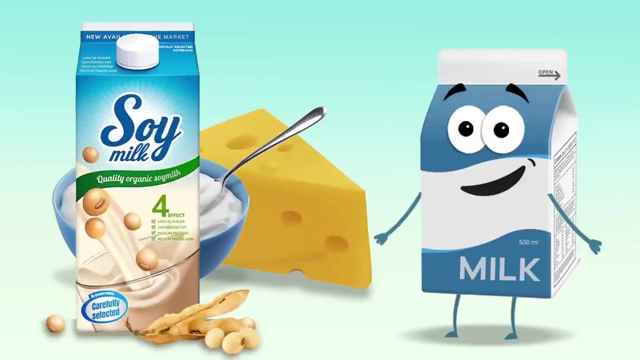 are also part of this group. Proteins are also part of this group. Our final food group is dairy, which, like proteins, goes beyond just milk, cheese and yogurt. Dairy alternatives like soy are also part of this group. Foods in this group provide calcium, a mineral good for. 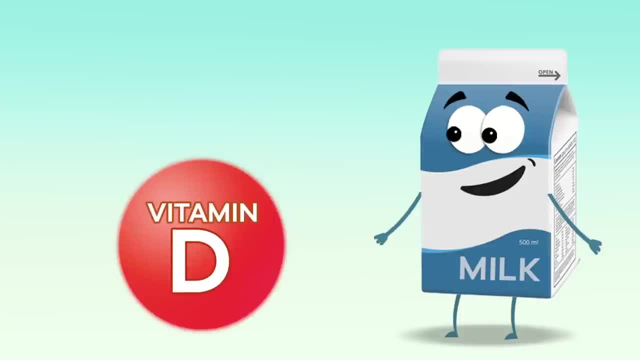 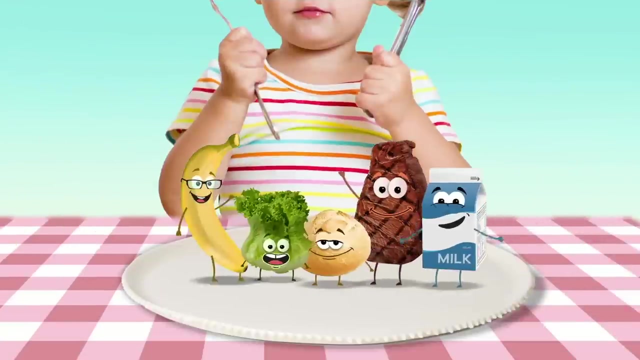 strong teeth and bones, and vitamin D, which helps your body absorb the calcium, reduces risk for diseases like heart disease and cancer and helps your muscles work correctly. To get an idea of what you should eat every day, let's play The Food Group Game Show. 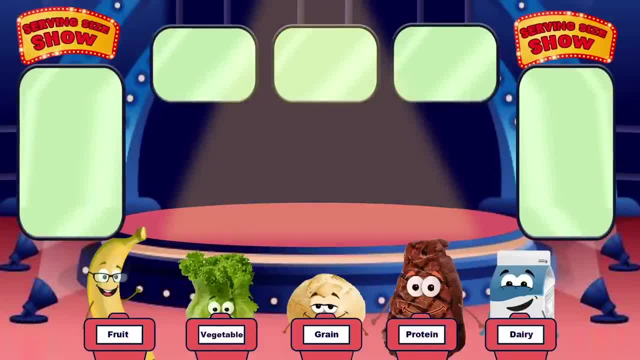 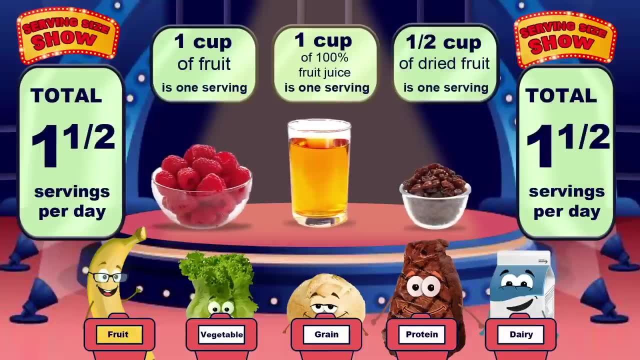 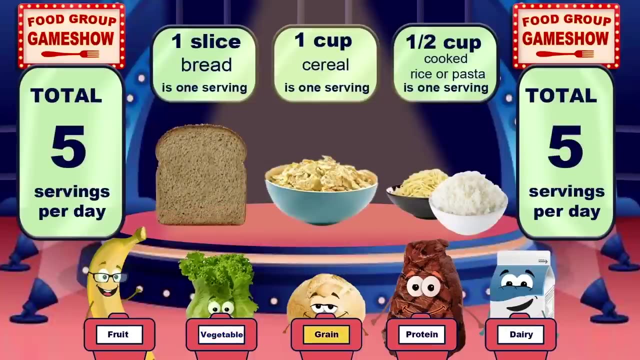 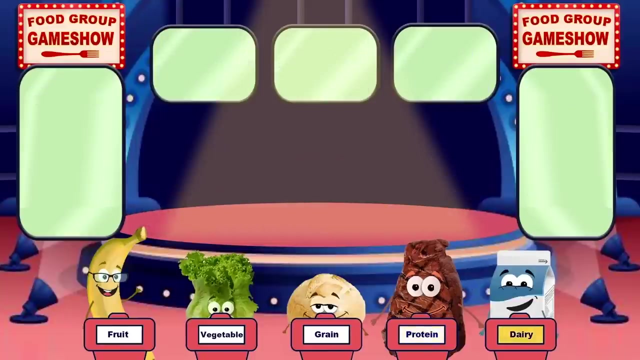 Here are some general guidelines on how much to eat from each group every day: Fruits: one and a half servings per day. Vegetables: two servings per day. Grains: five servings per day. Proteins: five servings per day Dairy: three servings per day. 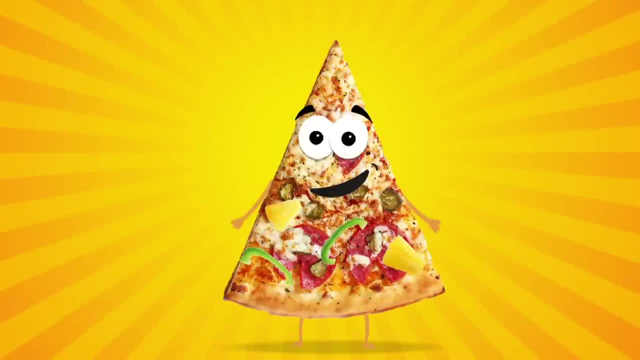 Some foods have multiple food groups in one, like pizza. A pizza can actually have all the food groups together in one place. For example, the sauce and veggie toppings come from the vegetables group. Pineapple as a topping comes from the fruits group. The cheese is from the dairy group. Meat toppings are from 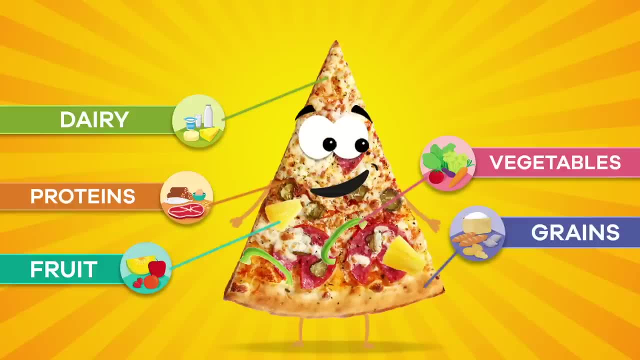 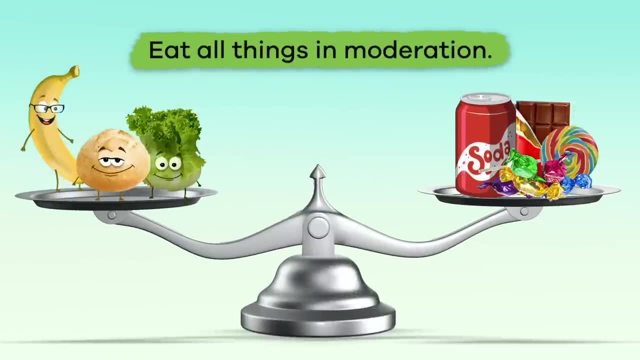 the proteins group And the crust is from the grains group. Impressive, right. The most important thing to remember is to eat the right amount of food in one place, To eat all things in moderation or in a balanced way. That way. 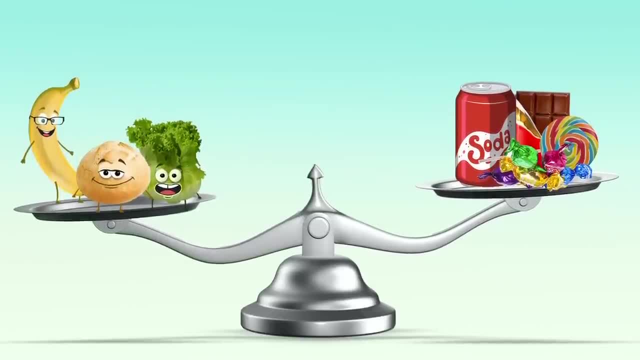 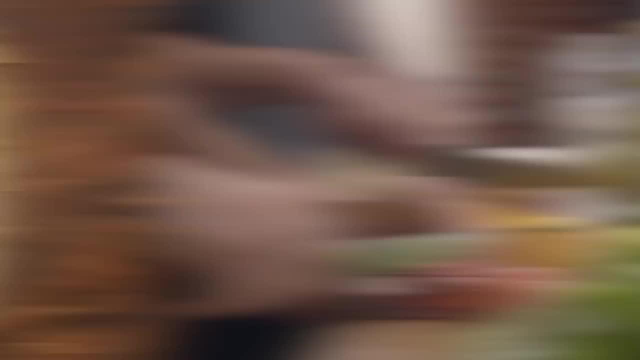 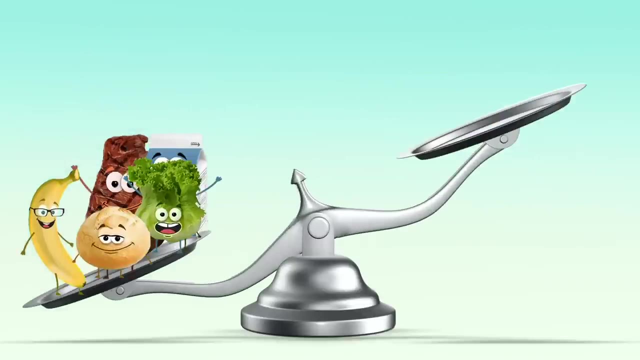 you are not having too much of a good thing, Literally. Treats like candy and soda are okay to have sometimes, but they do not have the same kinds of vitamins and nutrients as other foods. So try and limit how much candy and soda you eat.